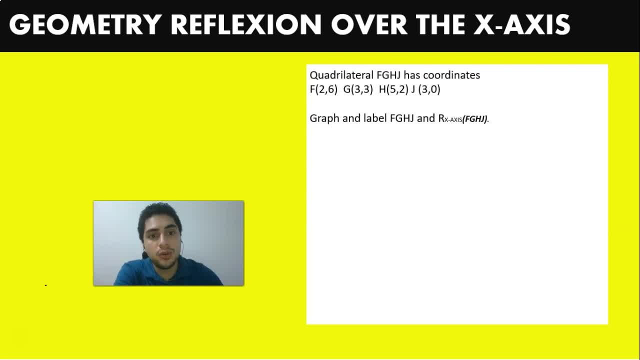 to graph that quadrilateral and its reflection over the x-axis: right. So now, guys, a real reminder: Whenever we have a point P and that point is reflected over the x-axis, the reflected point, so P- tick mark right is going to be x comma minus y, right? So whenever we have a point, 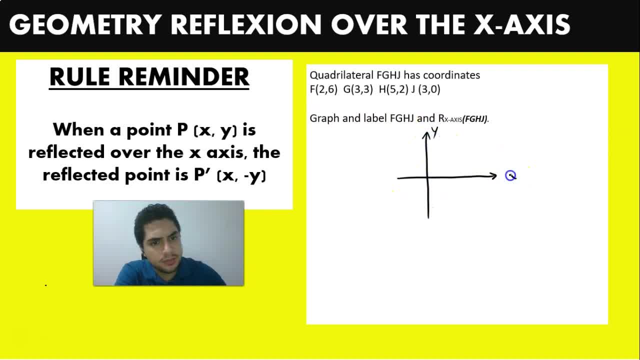 like, if we have our coordinate plane and now our x-axis is going to work as our reflection, it is as if we were, as if we had a mirror. The x-axis would work as it. so the x-axis would work as if it was a mirror, right? So in this, 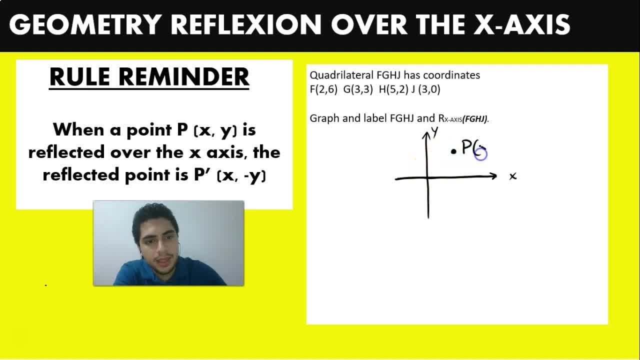 case, let's say we have a point here that has um coordinates, x, comma, y right. So this distance right is going to be maintained from the mirror and we're going to have our point And our new point. so P tick mark. 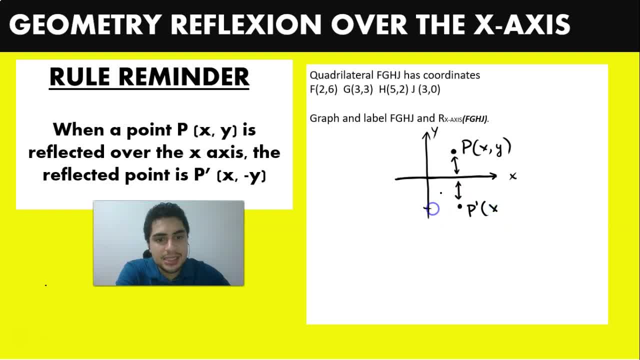 is going to have coordinates x and the distance, because it has to be the same distance from the point to the x-axis and to the x-axis to the new point, we're going to have the coordinate minus y. So whenever we are, 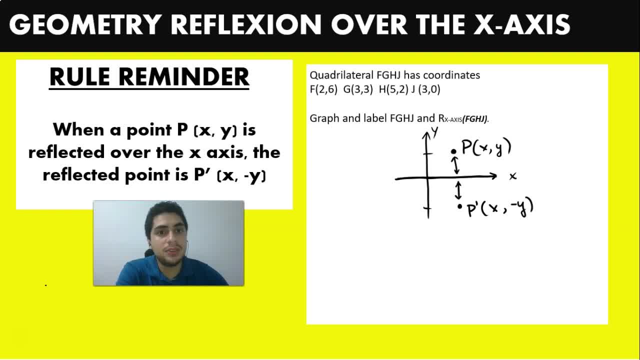 doing the reflection over the x-axis, we're going to have the same value of x but the opposite value of y, right? So in this case, the reflection over the x-axis of f g h y is gonna be f g h j. Sorry, Yes, So j. 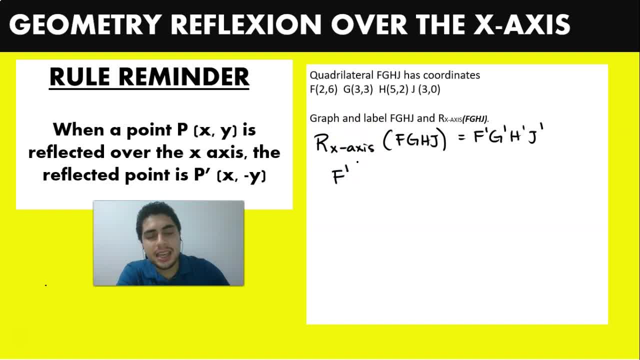 And now we have f is going to again have the same values of the initial value of f, So we're going to have 2, but then the value of y is going to be minus 6.. So we have g, and our new value of g is going to be 3, minus 3.. 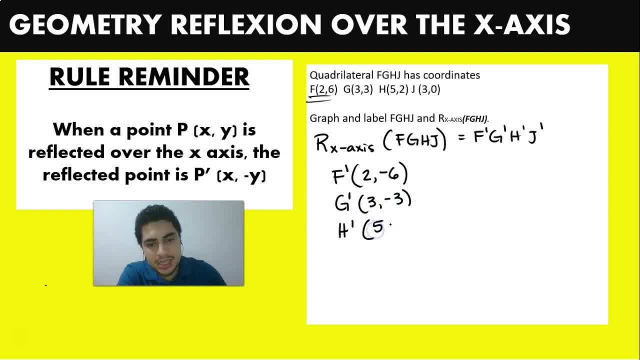 We have our value of h, We have the same initial value of x, but then the opposite value of y, And then, in the case of j, we have 3, and then the opposite of 0 is still 0.. And now what we're going to do is that we're going to graph points of f, g, h and j. 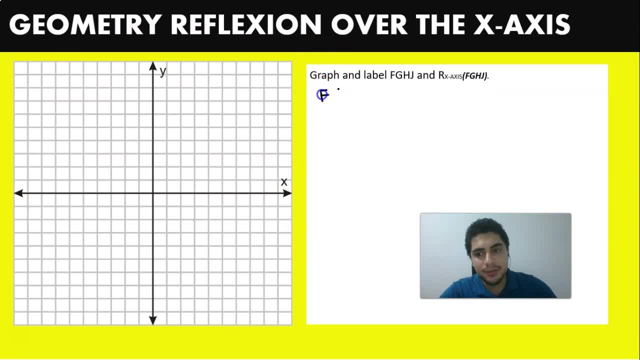 So we have the initial points, which are going to be f, which is 2, 6,, g, which is 3, 3.. We know that h is 5, 2.. And then we have g, which is 3, 3.. 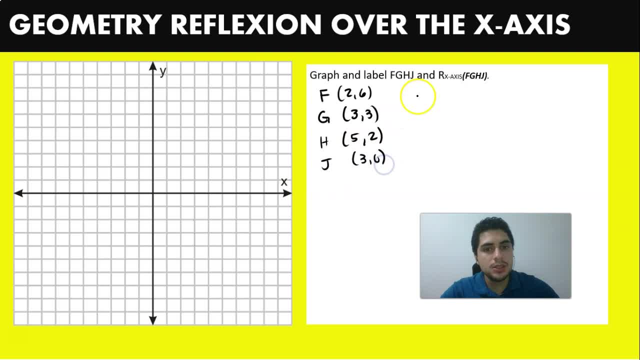 And then we have g, which is 5, 2.. And we know that j is going to be 3, 0.. We also know that our new points are going to be 2, minus 6.. g is going to be 3, minus 3.. 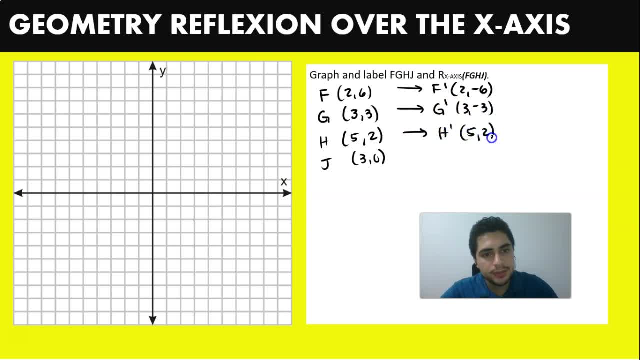 h is going to be 5,, 2, negative, And then we have that j is going to be 3, 0.. So now let's graph them. Now, f is going to be on 1,, 2, and 6.. 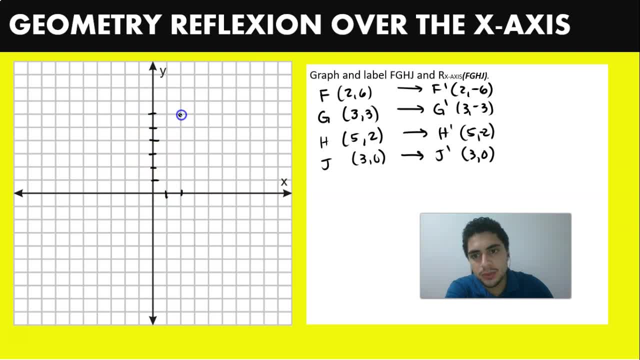 1, 2,, 3,, 4,, 5, 6.. So it's going to be here. g is going to be on 3, 3.. So 3, 3.. h is going to be on 5, 2.. 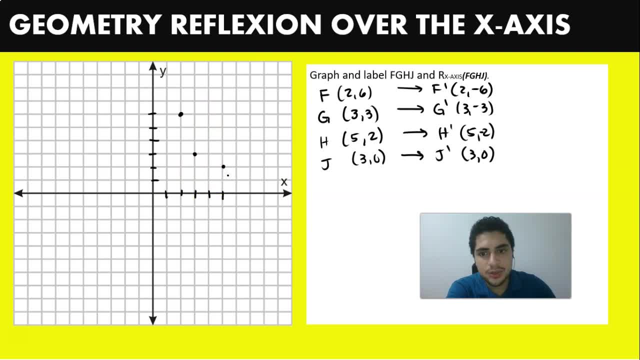 So 4,, 5, and 2.. And j is going to be on the value of 3, 0.. So it's going to be right here, Right? So our initial one is going to be here like this: 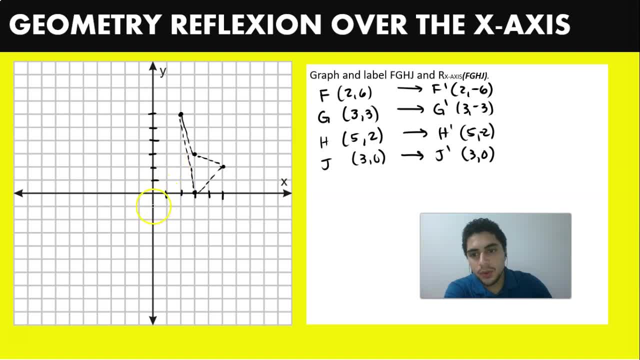 Now, in order to graph, we're going to have to do this. So, in order to graph the reflection, we're going to find f, which is going to be 2, minus 6.. So 1,, 2,, 3,, 4,, 5, 6.. 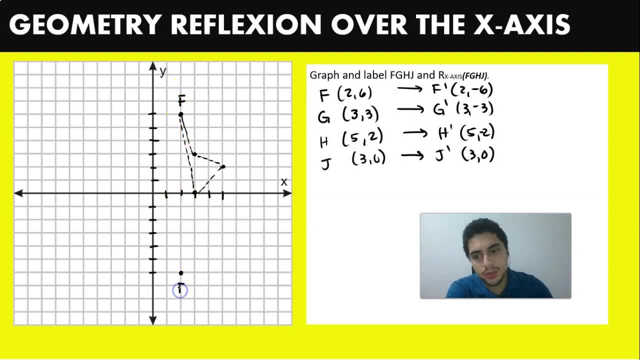 Right. So if before we had f, now this is going to be f. after the reflection, We have g, which is 3, minus 3.. So 3, minus 3.. So it's going to be here. We have our value of h. 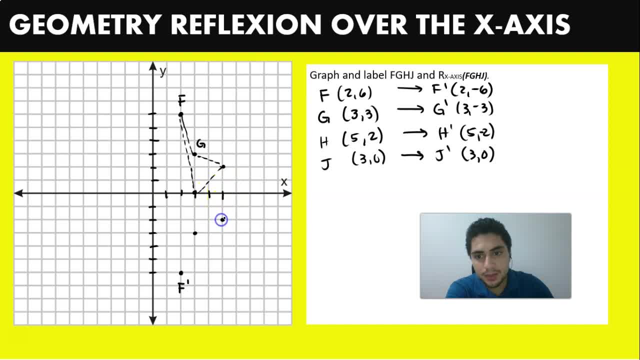 which is 9.. Now 5, minus 2.. So it's going to be here, And we have the value of j, which is still going to be 3, 0.. So we have g, h, We have h here.